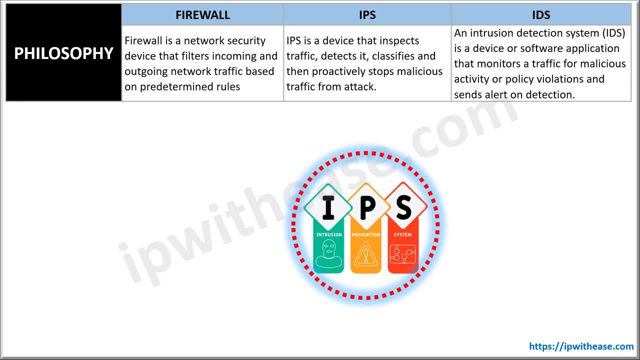 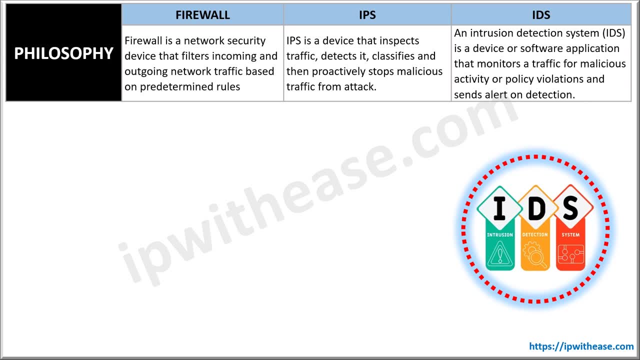 and then stopping the malicious traffic from attack. IDS is also a close relative of IPS. However, ITS will not block the traffic analyzed IPS. It will monitor the traffic for malicious activity and only sense the traffic. This alert is generally sent either to the network or security administrator, or else. 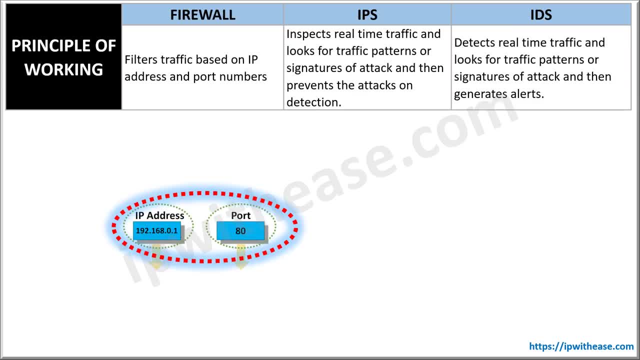 to a SIEM system. A firewall allows traffic based on a set of rules configured. It relies on the IP source, IP destination addresses and the ports. A firewall can deny any traffic that does not meet the specific criteria. IPS inspects real-time traffic and looks for the traffic pattern and signatures Based. 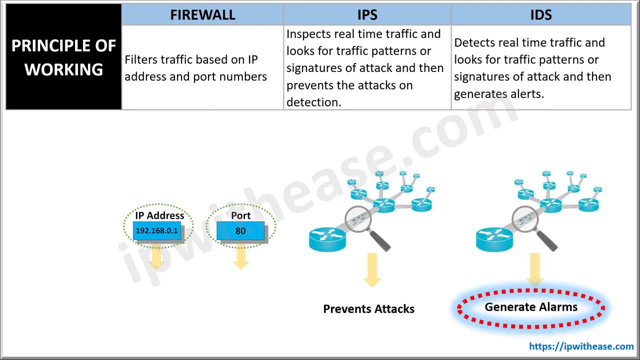 on its detection, it will prevent the attack. IDS will also detect the anomaly with SIEM approach. However, it will send the alert and not disrupt the traffic. Here it is important to note that IPS can sometimes give false positive results and block a legitimate traffic. 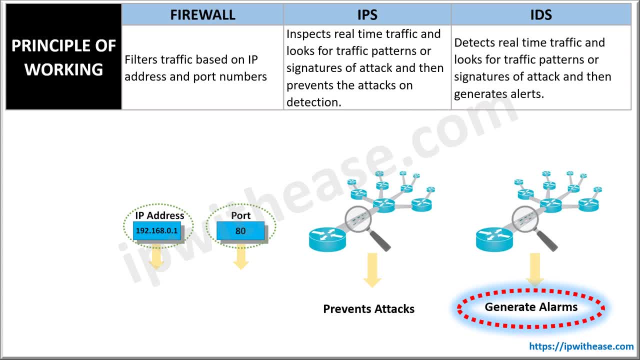 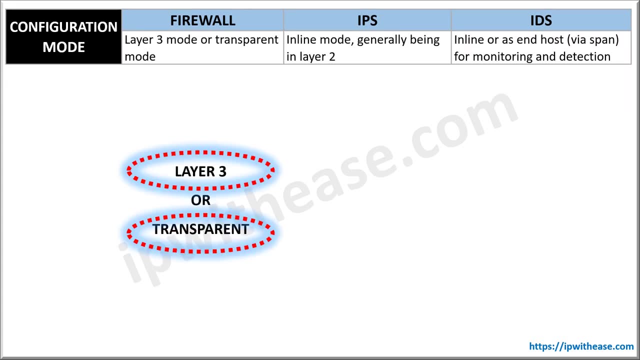 So let's see how it works. Hence many administrators or companies prefer to have IDS in the setup and not IPS, since they don't want the genuine traffic to be blocked, which can be a bad customer experience. In terms of configuration mode, firewall is configured in inline layer 3 mode or transparent. 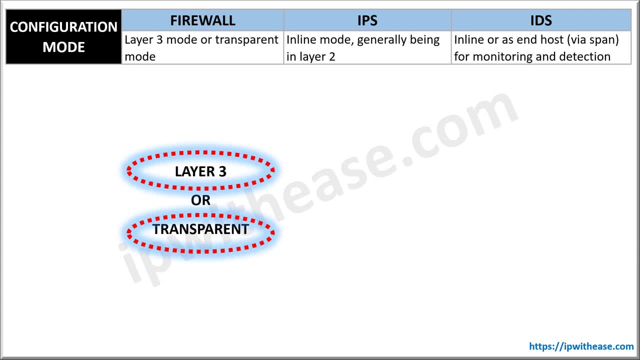 mode. In layer 3 mode it is required to have separate segments carved out and the network, or to be precise, arc grid, checked. However, transparent mode is simple to implement with no significant changes in network, albeit there are some associated limitations in transparent mode. 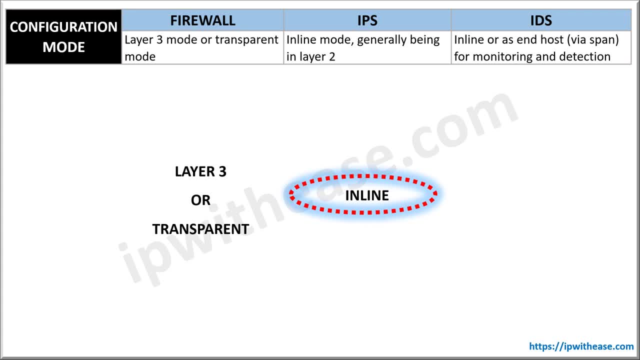 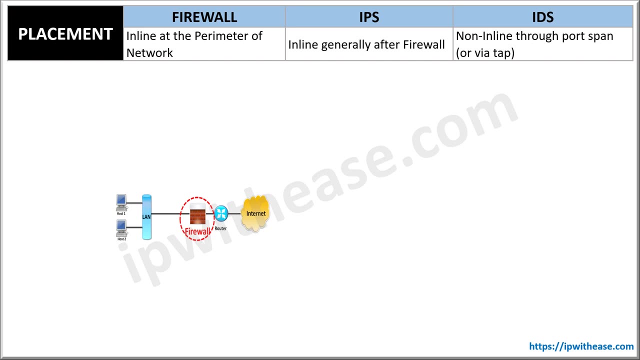 Talking about IPS, it always has to be in inline mode, while IDS can be either in inline mode or the host, that is, spam mode. When it comes to placement of these security devices, firewall is placed at the perimeter or edge of the network, which is much closer to the 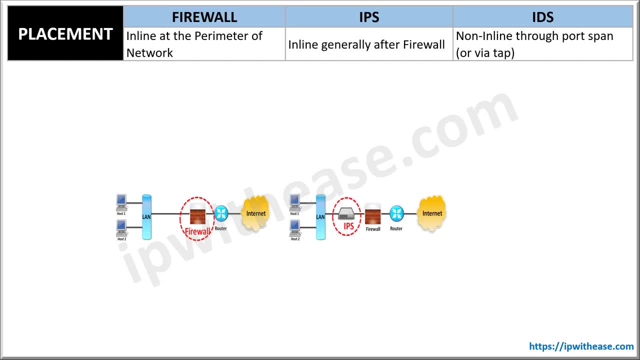 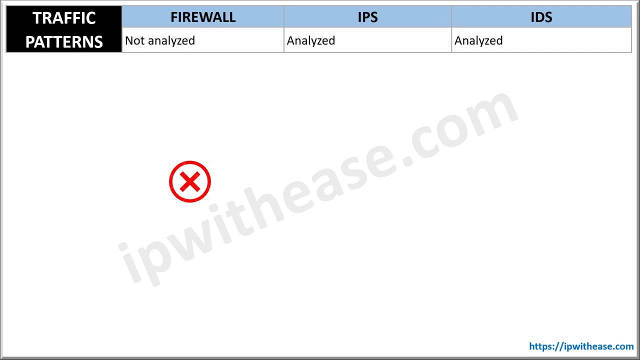 internet entry exit points. IPS also should preferably be provisioned after the firewall, and then IDS can be positioned in non-inline mode. that is also called spam mode. A very interesting distinction of firewall from other two elements is that firewall doesn't analyze traffic patterns. 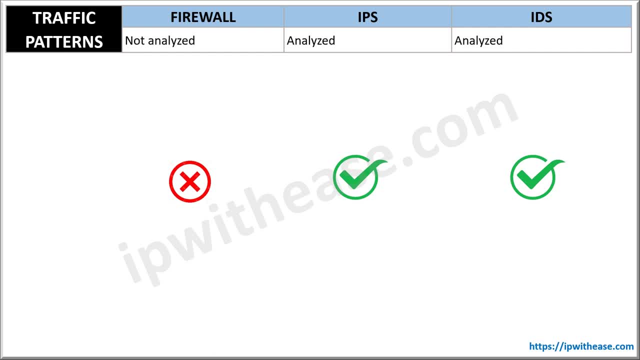 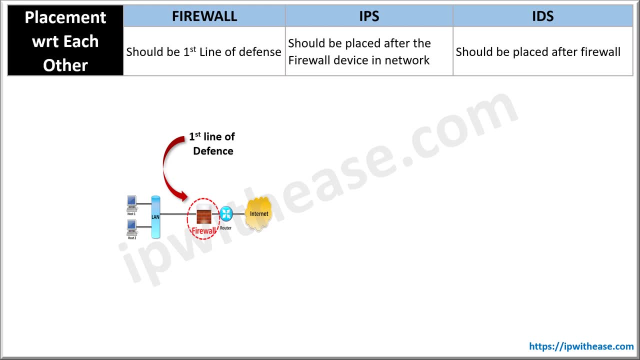 While IPS and IDS have the key functionality to analyze the traffic flow or patterns, As we discussed earlier, firewall is always first line of defense. IPS should be placed after firewall When it comes to action taken on detection of unauthorized traffic. firewall simply blocks. 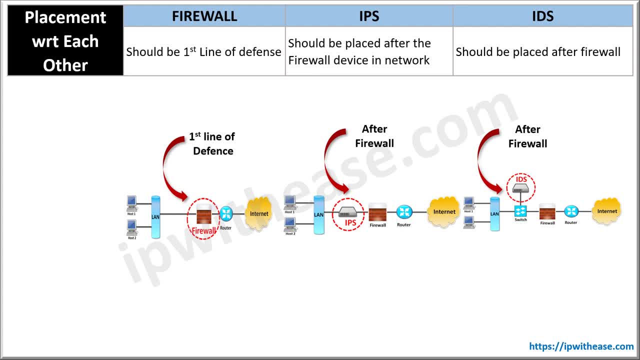 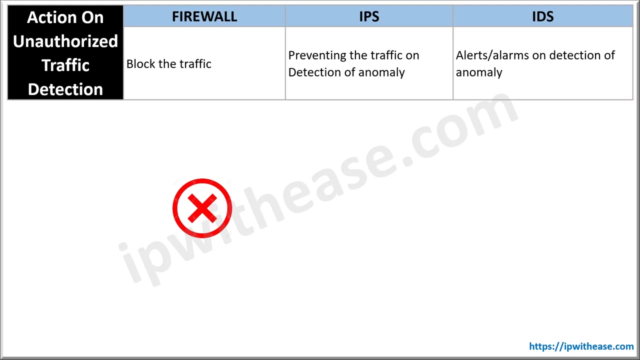 the traffic from entering, and same is what IPS will do. However, IDS will not prevent the traffic from entering the network, rather just sends alert to the concerned. and same is the case of IDS, which should analyze the traffic after the firewall When it comes to action taken on detection of unauthorized traffic. firewall simply blocks. 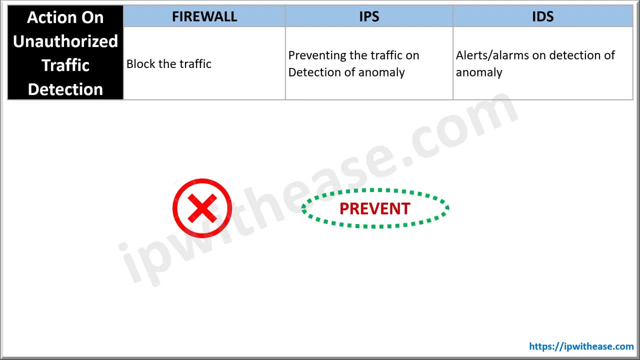 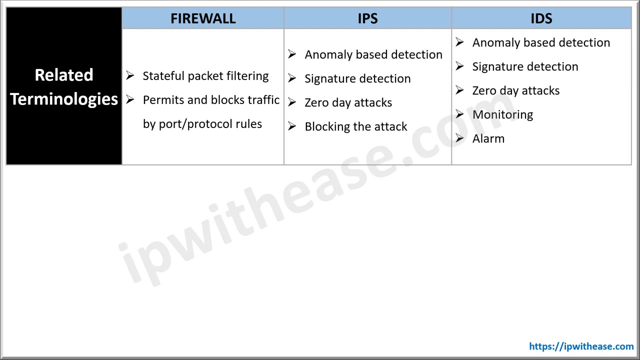 the traffic from entering, and same is what IPS will do. However, IDS will not prevent the traffic from entering the network, rather just sends alert to the concerned. Now that we have high level understanding of the three essential security components, let's reiterate the key features and functionality of each one. 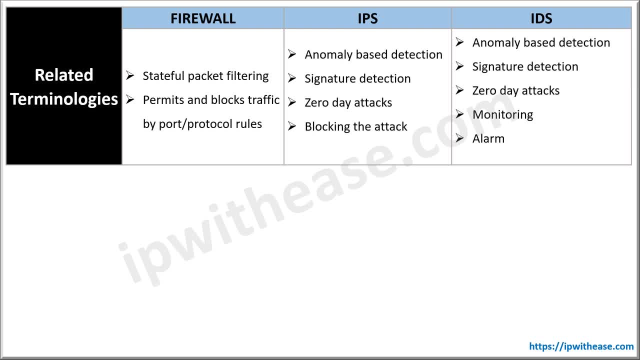 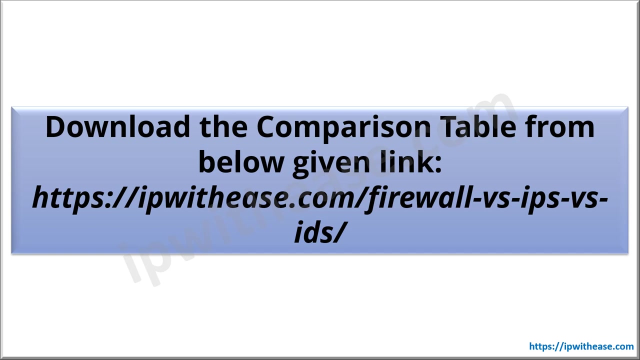 Firewall. related terms are stateful firewall, filtering and inspection. It permits and blocks traffic based on ports and protocol rules. It permits and blocks traffic based on ports and protocol rules. It permits and blocks traffic based on ports and protocol rules- iphssä. That's it from the comparison of security components, ie firewall, IPS and IDS. I hope. 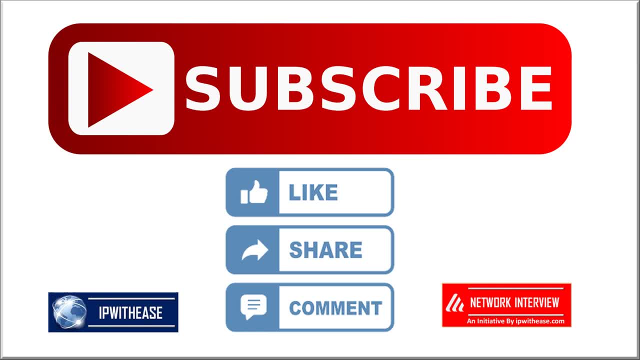 you liked this crawl video and please don't forget to like and subscribe. thank you.